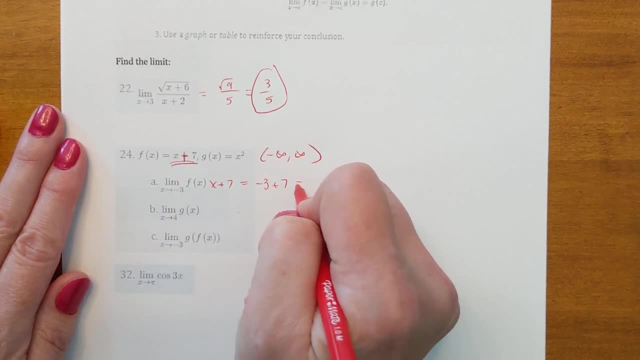 So when you plug in negative three, you get negative three plus seven, which is four. For g of x, it's x squared. So plugging in the number four, you get four squared sixteen. All right, g of f of x. 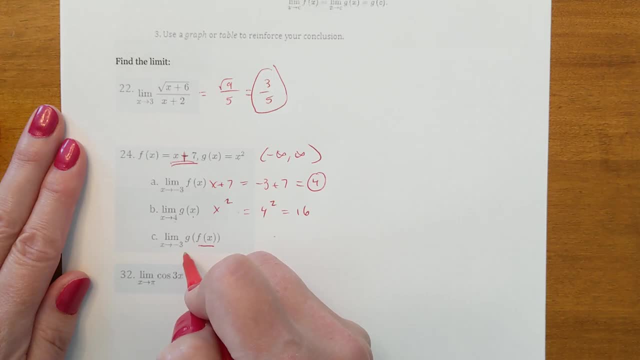 Well, we had just found f of x as it approached negative three, So as it approaches negative three, we got four. So that is equal then to the limit, as x approaches negative three, Of g of four. So then g of four, putting the four in for g. we already did that and we got sixteen. 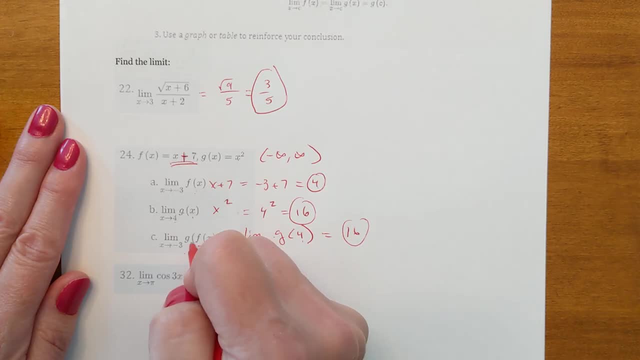 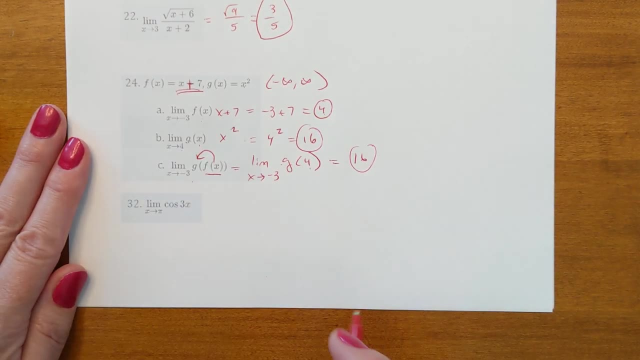 All right. so remember, when you're doing g of f, you have to start with the inside nest and plug it into the one that's to the left. Okay, cosine is also has an infinite domain, from negative infinity to infinity. 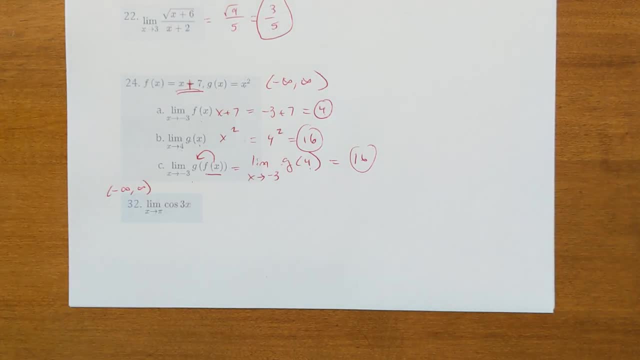 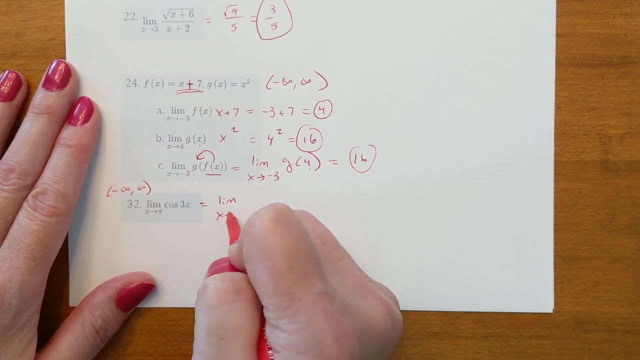 It is defined for all x. It's a continuous, It's a sine wave, Sine cosine wave. So anyway, when you plug the pi in, you get the limit as x approaches pi of the cosine of three pi. Remember, cosine repeats every two pi. so we can subtract off, we can take off two pi. 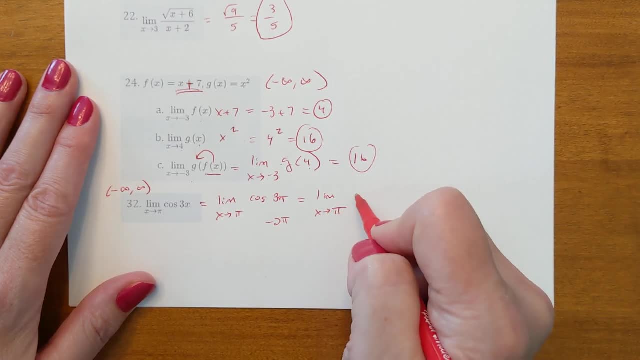 from it. So it's really the limit, as x approaches pi, of the cosine of pi. Three pi minus two pi is one pi, And so hopefully again you're remembering what it looks like visually in your head. It starts and ends at one. 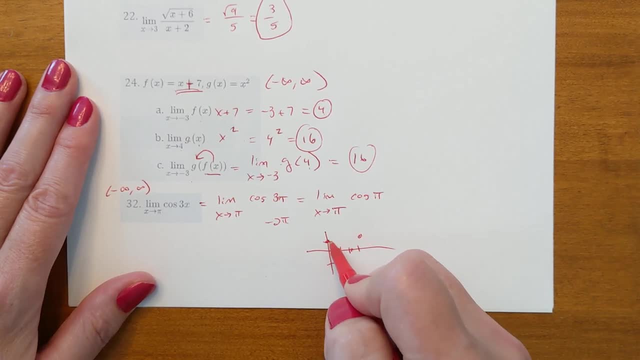 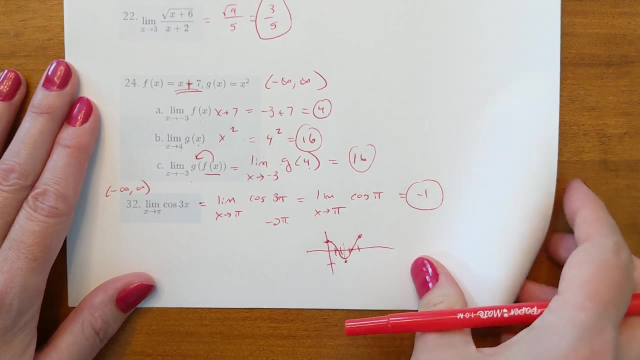 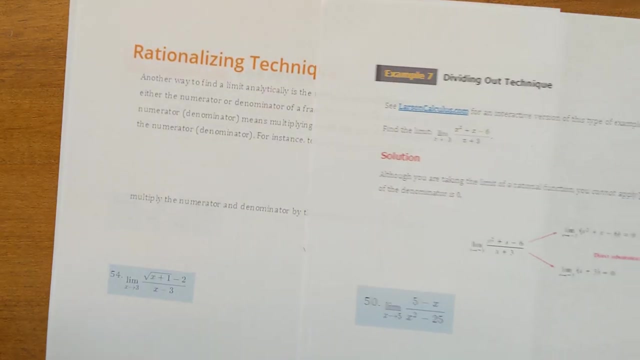 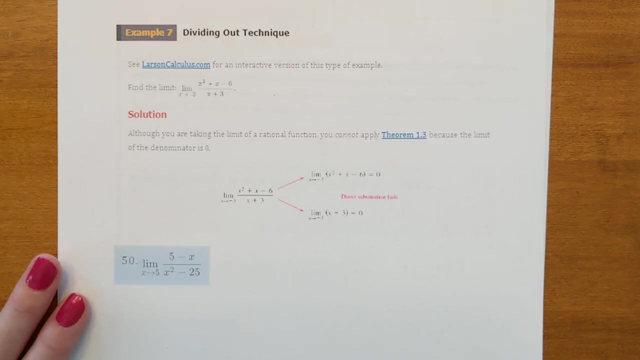 In the middle. at pi, it's down at negative one, Then it goes through zeros. So when it's pi, it's down here at negative one, All right. Sometimes, though, it's going to be undefined, And when it's undefined, we're allowed to divide out where it's undefined at, and then 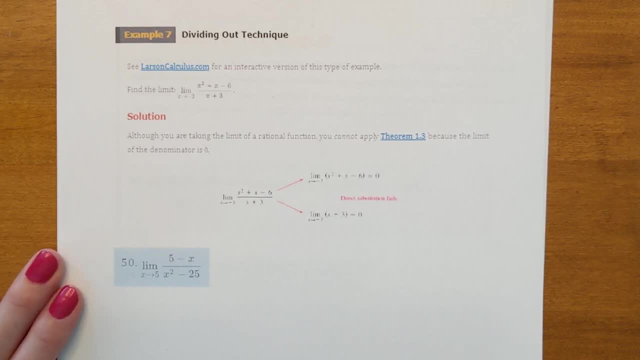 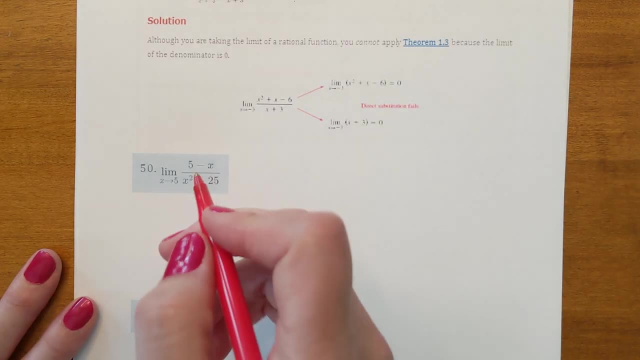 continue on from there. So it's called the dividing out technique. So let's do that on one of them here. Now, if we plug five into this, it's going to be undefined, because you'd have five squared minus 25, or 25 minus 25,, which is zero. 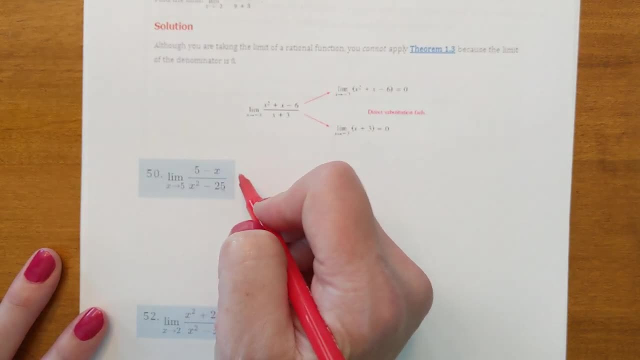 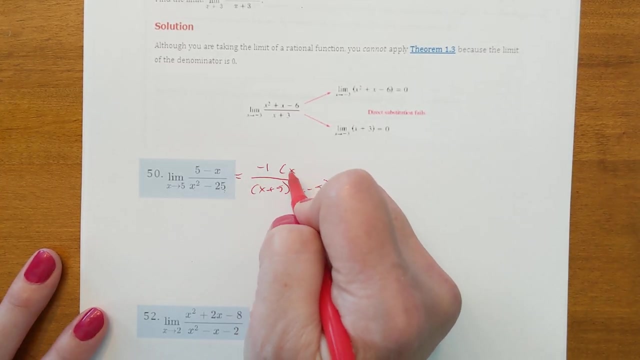 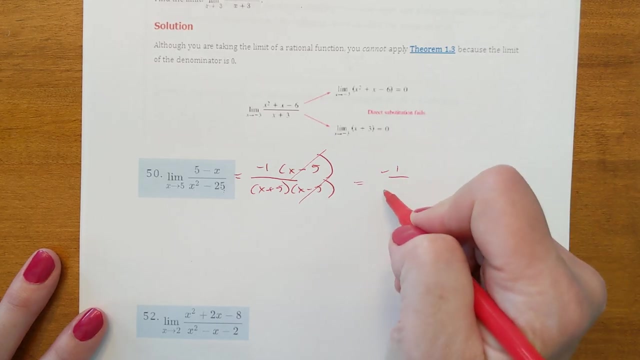 So you can't do that. But we can factor in the top and the bottom. The bottom factors into x plus five times x minus five And the top, if you take out a negative one, it factors into an x minus five. So we can cancel out the x minus five, which leaves negative one over x plus five. 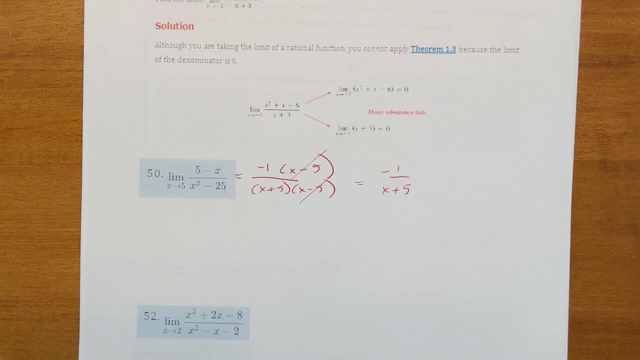 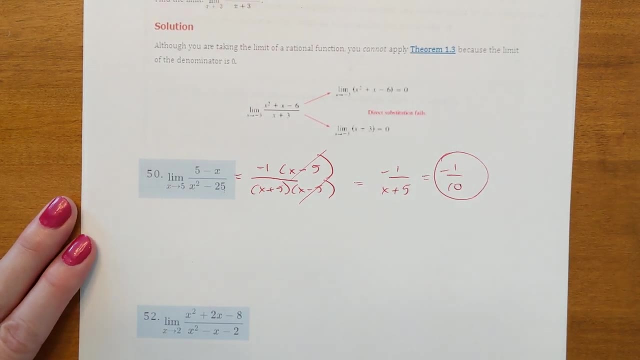 That's called the dividing out technique. Now when you approach the number five, when you put the five in there, you get negative one over ten. So it approaches the number negative one-tenth. Same thing on next one, on number 52.. 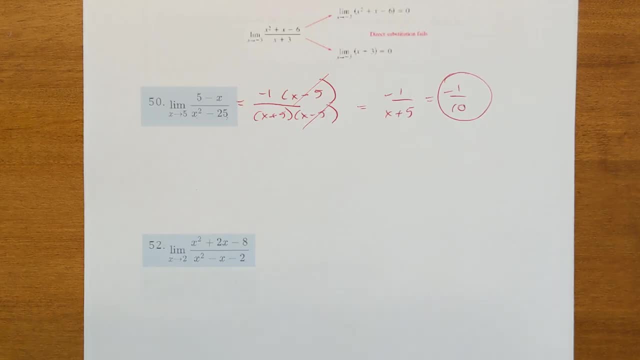 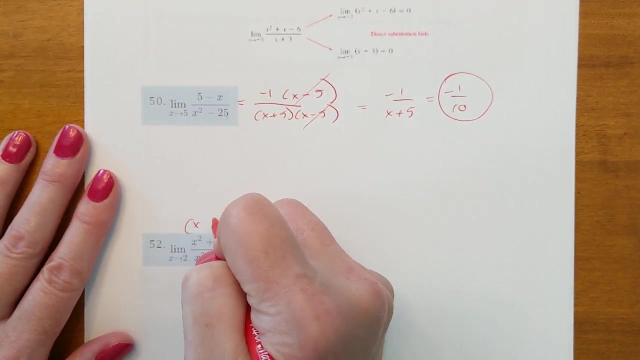 We can factor that. So the top of it factors into: let's see here: Ah, I don't see it, That's okay, I can do it myself. So the top of it factors into: let's see x and x, four and two. 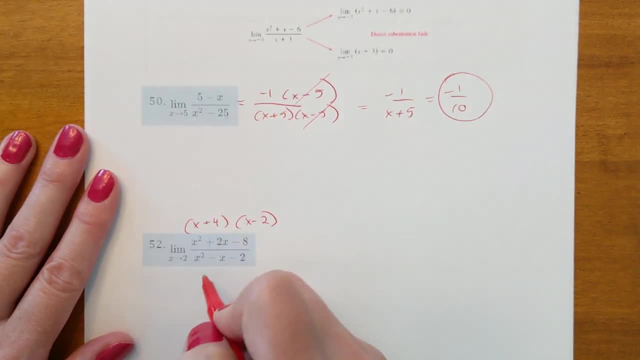 We want it to be a positive two, so it's plus two and minus two, And on the bottom, two times one. We want it to add up to a negative one, so we want it to be two negative and that one positive. 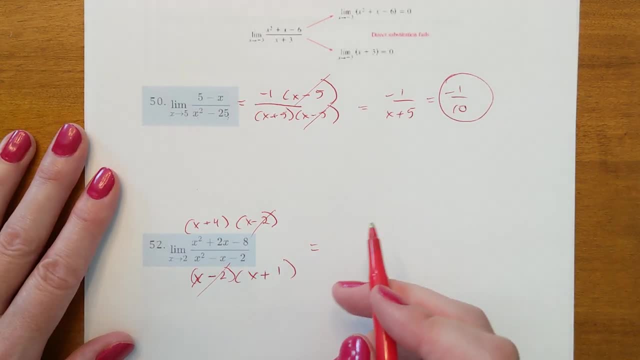 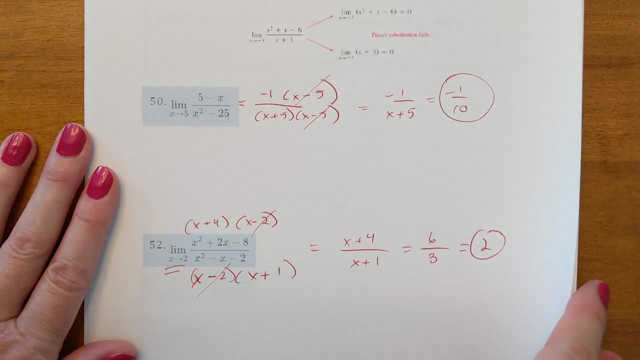 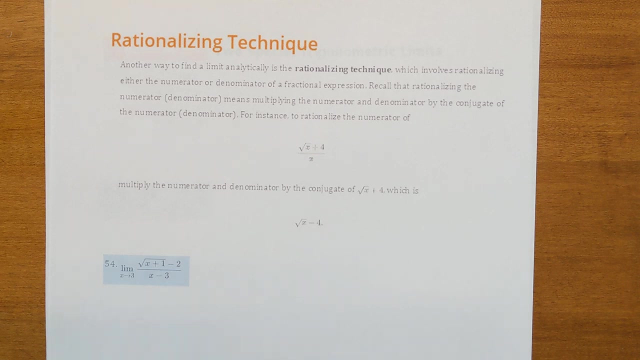 So the x minus two cancels out which is good. So that leaves you with x plus four over x plus one. So when you divide, when you substitute in, then x equals two. it gives you six over three or two, And then sometimes you have a real mess, and so what you can do is rationalize it by multiplying. 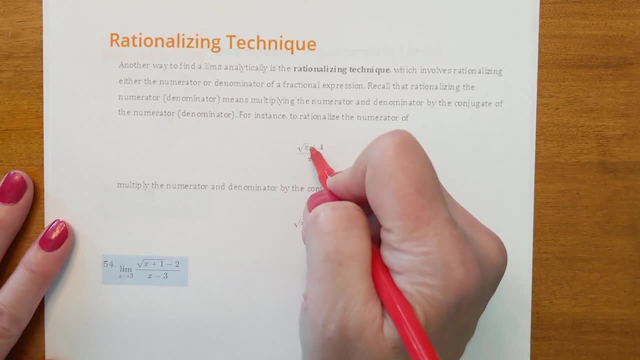 the top and bottom by the conjugate of it. So here you got the square root of x plus four, So the conjugate of it. remember you used the opposite sign. so instead of plus, you're going to multiply by the square root of x minus four. on it. 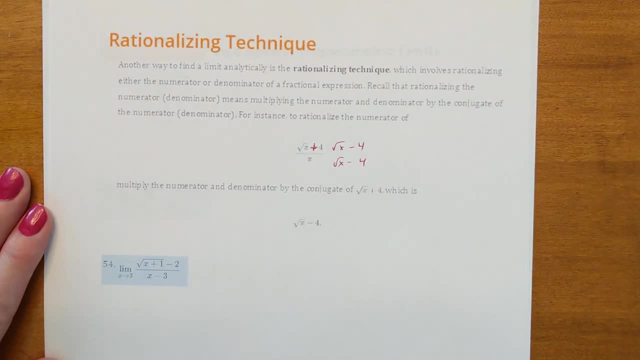 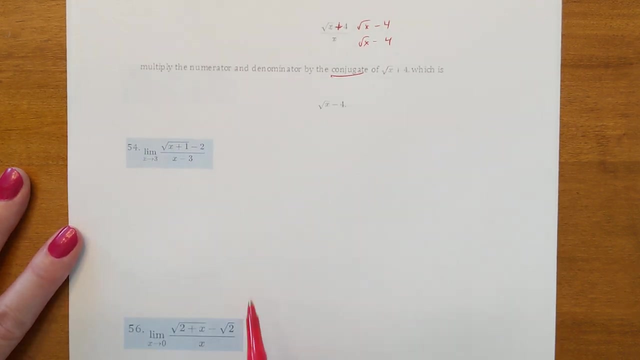 That's what the conjugate of conjugate of it is. Or if it would have been minus, you would multiply by a positive four. So well, it's called rationalizing, All right. so by multiplying by the conjugate, All right. so down here we're going to rationalize it. 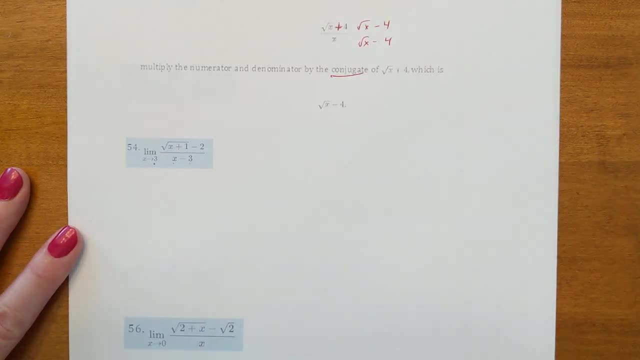 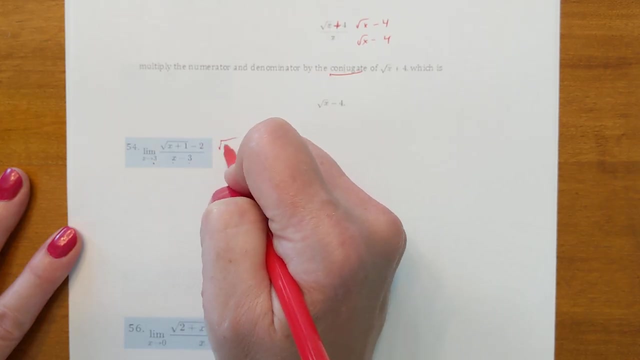 If you plugged in the number three, you'd have three minus zero, undefined. so you can't just plug it in. So what we're going to do is rationalize it by multiplying by the conjugate. It's minus, so we're going to multiply by the opposite plus on the top and the bottom. 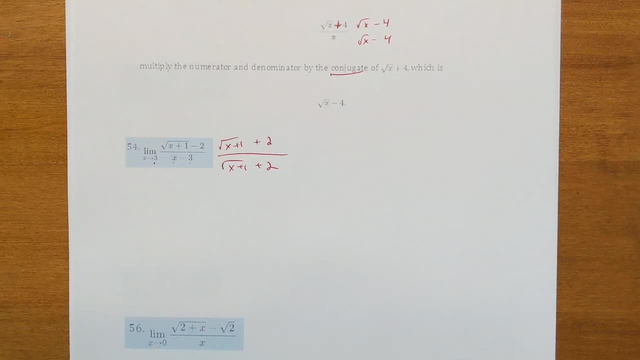 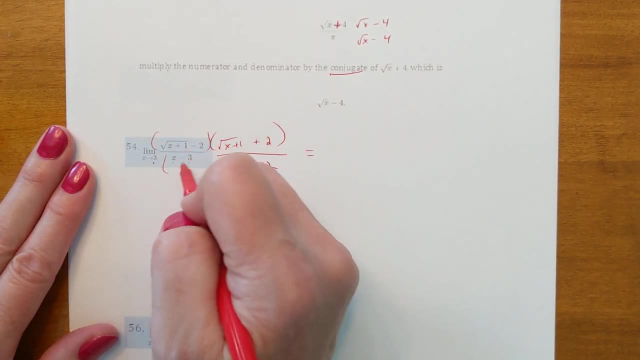 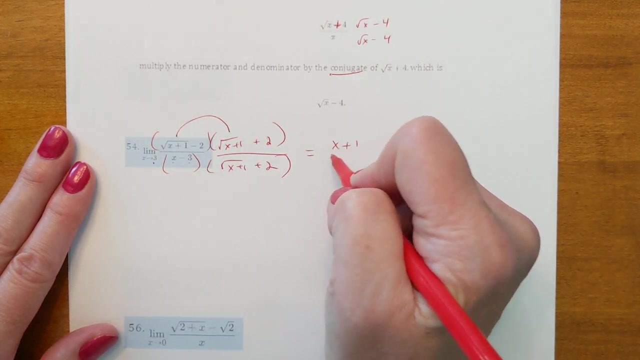 So it's like you haven't done anything because you're multiplying the top and bottom by the same fraction, so it's not a big deal. So on the top you're multiplying the whole thing by it. So square root of x times plus one times, the square root of x plus one is x plus one. 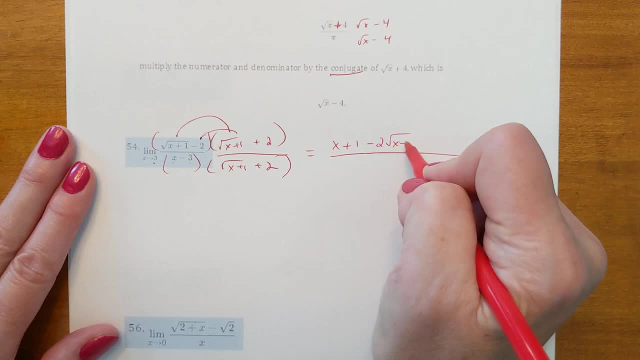 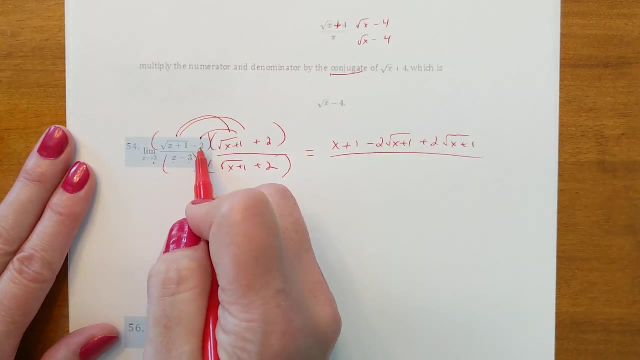 And then the middle. here you have negative- two times the square root of x plus one, plus negative- two plus 1, and on the outer you have 2 times plus 2 times the square root of x plus 1, and then negative 2 times positive. 2 is negative 4, and then in the denominator- let's start with 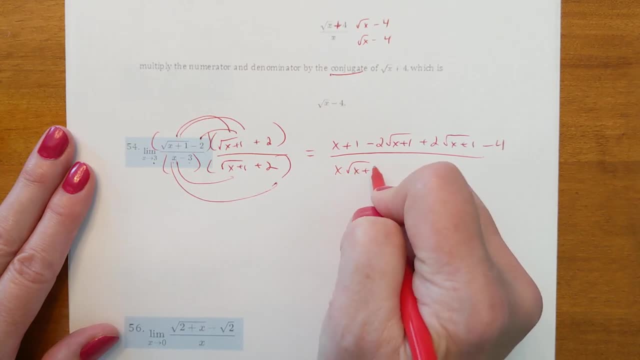 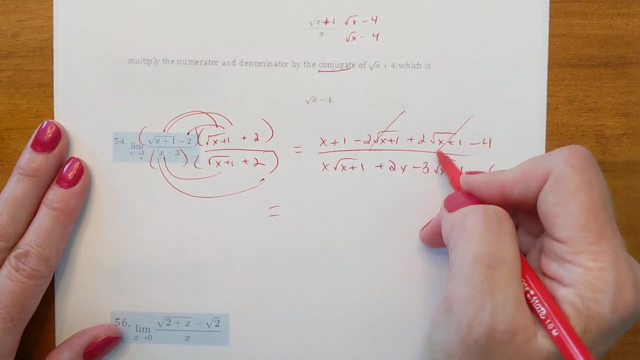 the x, so x times the square root of x plus 1, then x times plus 2, then on the inside you have minus 3 times the square root of x plus 1, then minus 3 times plus 2, minus 6, alright, so from doing all that, it cleans up, that's gone because it's minus and plus. 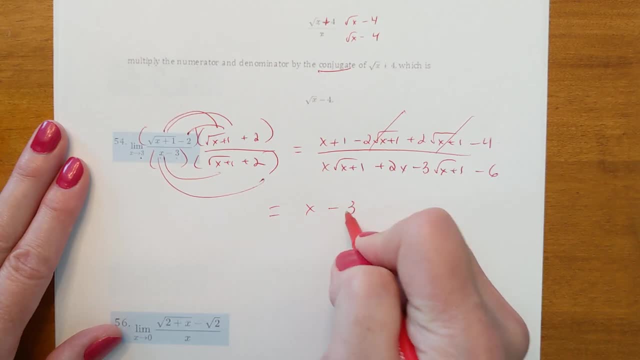 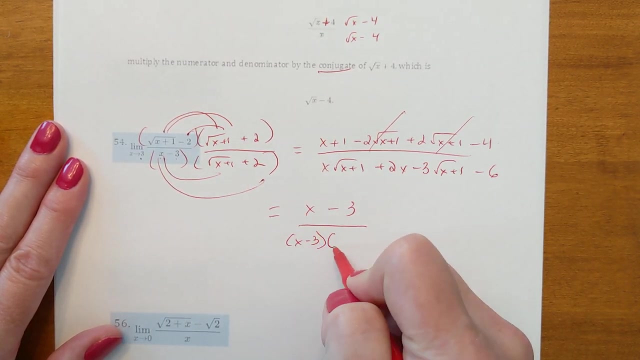 so on the top, you're left with x minus 3, and then down on the bottom, in the denominator, what you're left with, you know what? I think we probably should have just left it alone. yeah, if we would have just left it alone, we have x minus 3 times that whole chunk there. 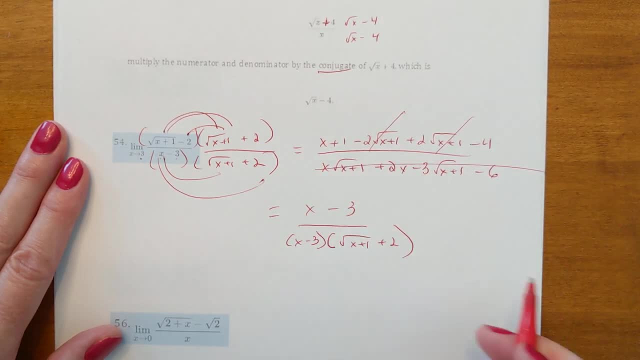 the square root of x plus 1 plus 2, we didn't need to do all that. So that's it. So that's it, So that's gone. and then you're left with 1 over the square root of x plus 1 plus 2.. 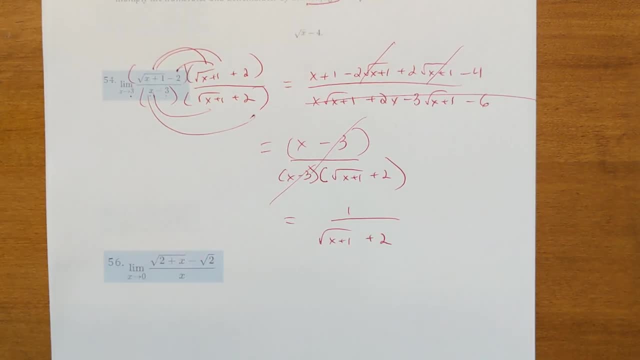 Alright, sorry, I over chewed on that, I'm sorry. Okay, so we're still trying to find the limit, though, as x approaches 3, so now that we've rationalized it, you can just plug the 3 in. 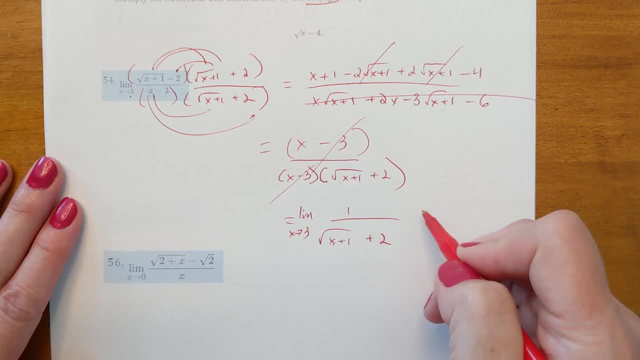 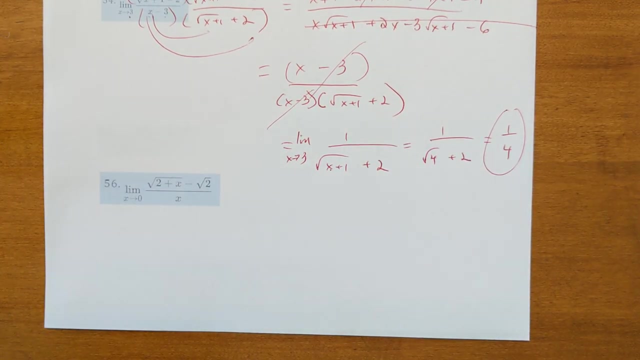 So the limit as x approaches 3 is 1 over the square root of 4 plus 2, so it's 1 over. let's be clear: 1 over 2 plus 1 plus 3 times x, so that's just 1- 4.. 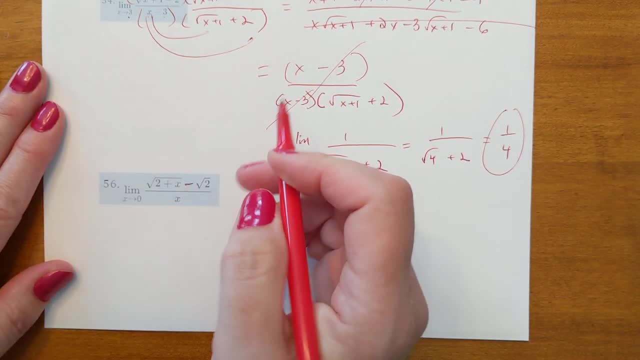 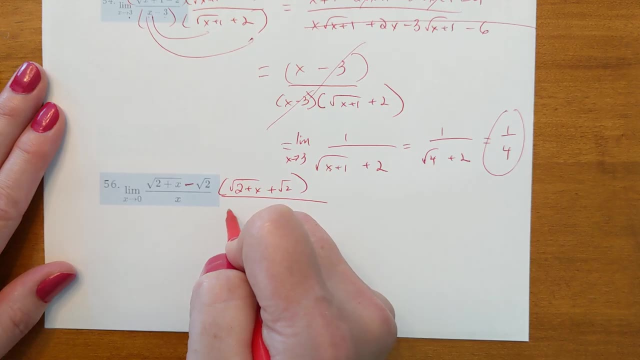 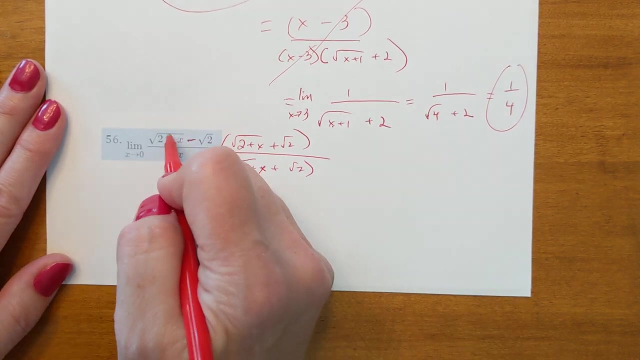 Alright, next, one same idea. same idea: you're gonna multiply by the conjugate. so instead of minus, I'm gonna multiply by a plus. So the square root of 2 plus x plus the square root of 2 over the square root of 2 plus x. 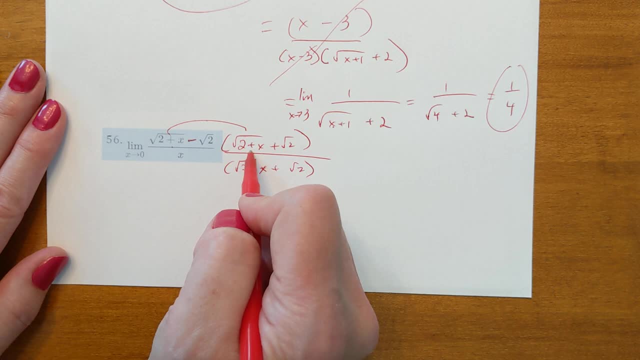 plus the square root of 2.. Alright, so on the top, the square root of 2 plus x times the square root of 2 plus x is just 2 plus x. So what we've done is we've just x plus 1 plus 2 is equal to the x plus 4, so that's. 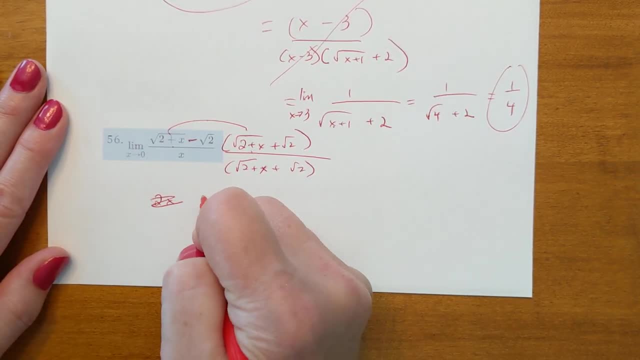 the square root of x. Okay, so we've just x and then x, And now we're gonna talk about the square root of x plus 2, so let's, And then square root of 2 plus x times the square root of 2 would be plus the square. 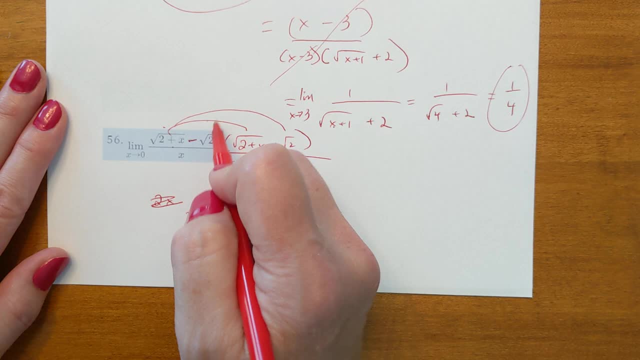 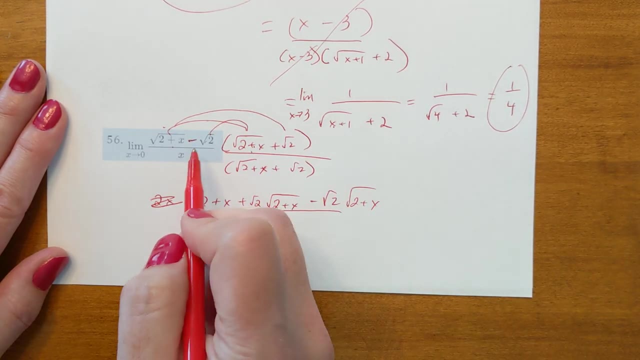 root of 2 times the square root of 2 plus x. Now do the negative 2.. So negative 2 times it is minus the square root of 2 times the square root of 2 plus x, And then negative square root of 2 times positive square root of 2 is negative square root of. 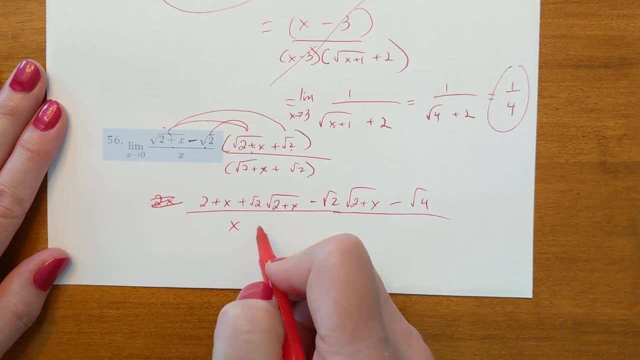 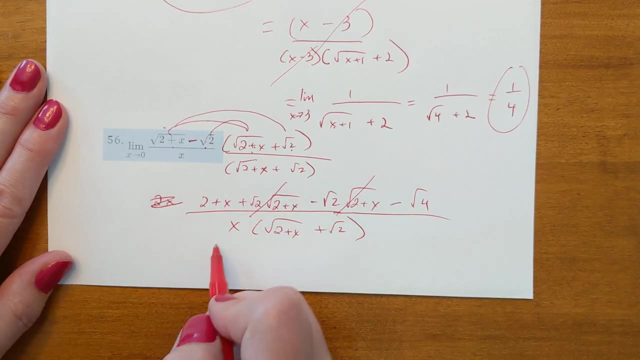 4.. And then on the bottom, I'm just going to leave that alone. I forgot to leave it alone. Sorry about that. Okay, so on the top, that's gone and you have x and that square root of 4 is 2.. 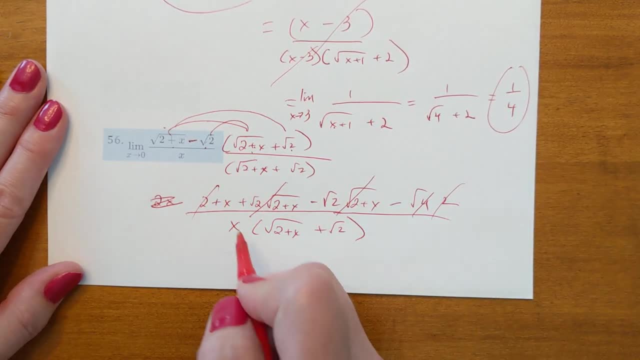 And so you have minus 2 plus 2, they're gone. So you have just the letter x left on the top, Over on the bottom, x times in the chunk here, square root of 2 plus x plus the square root of 2.. 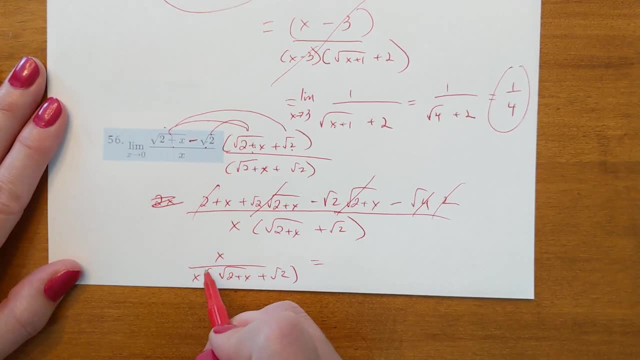 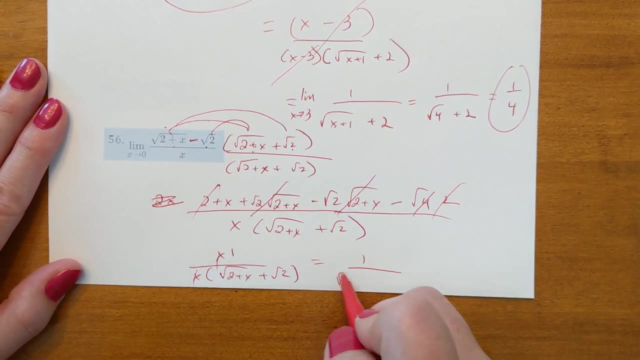 So you can cancel that out. Now you be careful: When you cancel the x out here. you have to leave the number 1 out. 1 on top, because this is in the denominator. It's going to stay in the denominator. It doesn't float up magically because you've canceled out the letter x's. 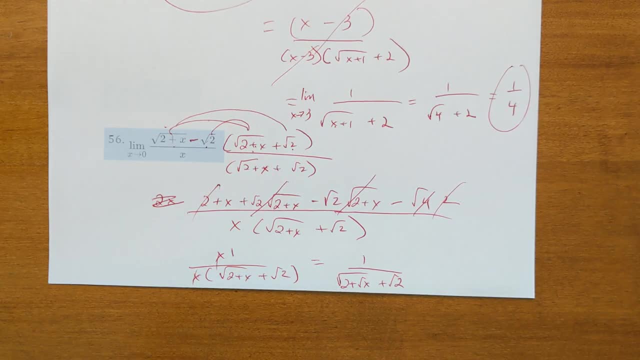 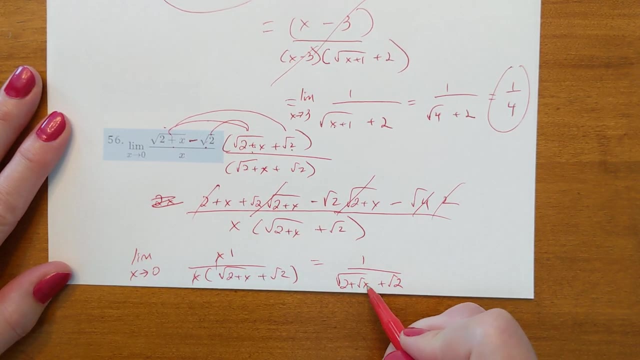 It stays in the denominator. So we're finding the limit again is x approaches 0 of all of this. So now we can just plug in. oh, I made a mess there, didn't I? Now we can just plug the 0 in, so that gives you 1 over the square root of 2 plus the square. 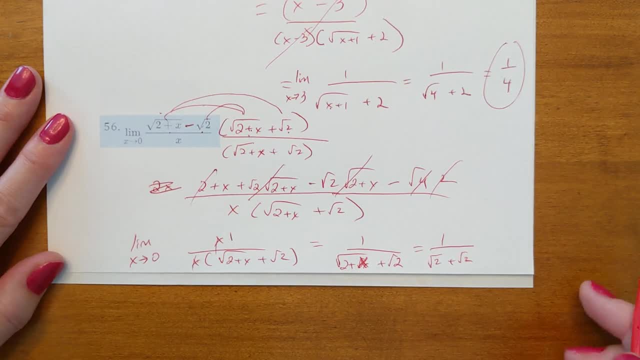 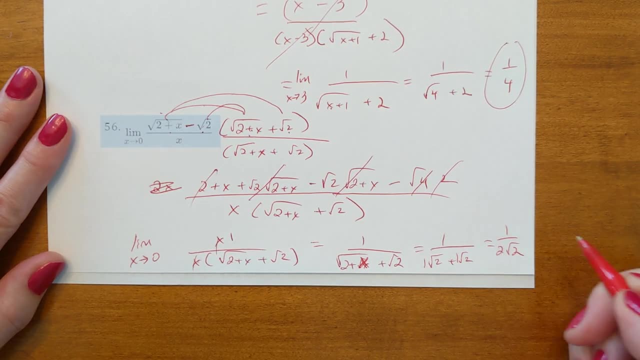 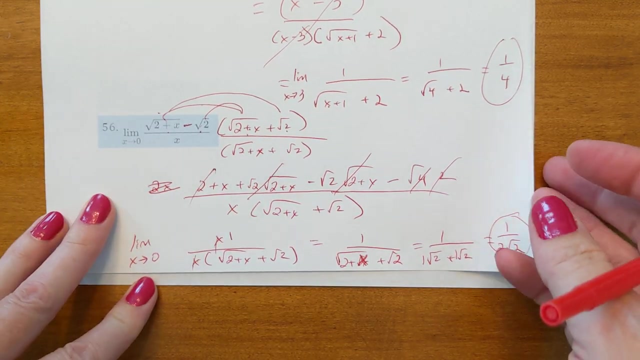 root of 2.. So when you do that, you end up with the square root of 2, 1 of them and plus another one of them, You get 1 over 2 times the square root of 2.. So that's the answer. 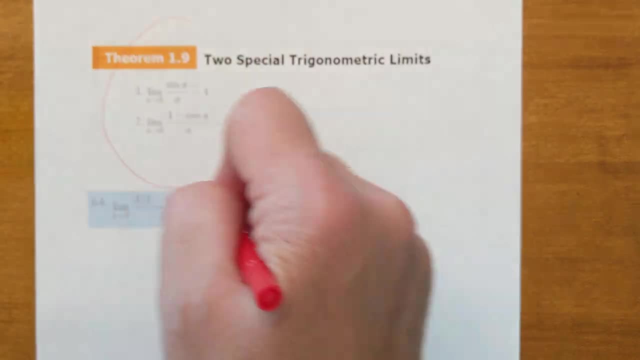 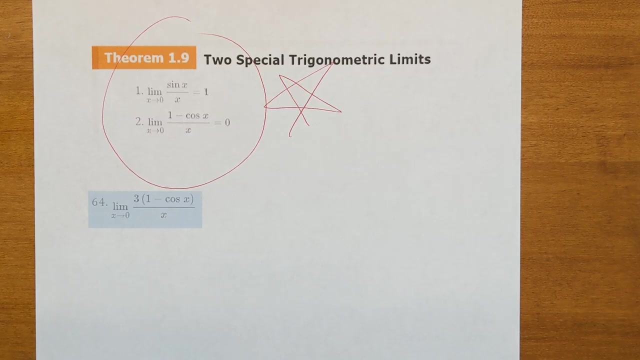 And then there's a couple special trigonomic values that you need to memorize, So make yourself a flash card. The limit, as x approaches 0, of the sine of x over x equals 1. over the square root of x equals 1. all the time.